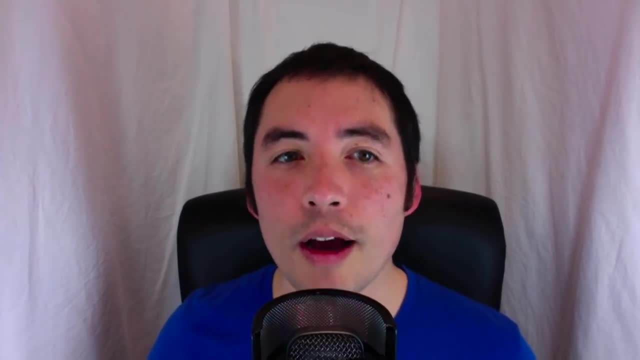 this one doesn't have a simple answer and there are books about feature selection, I assume, but it's certainly a book-length topic. But I think the best way to answer this is: two years ago I was at Pi Data DC in Washington DC and I attended a presentation called. 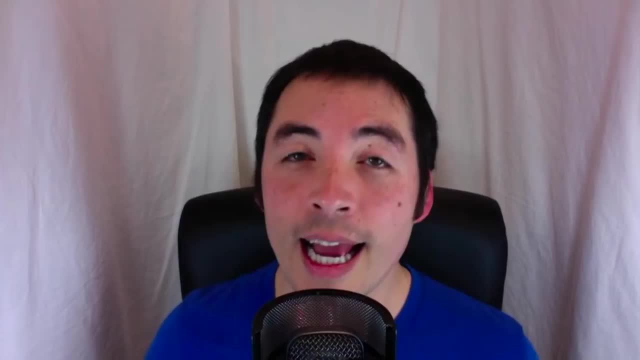 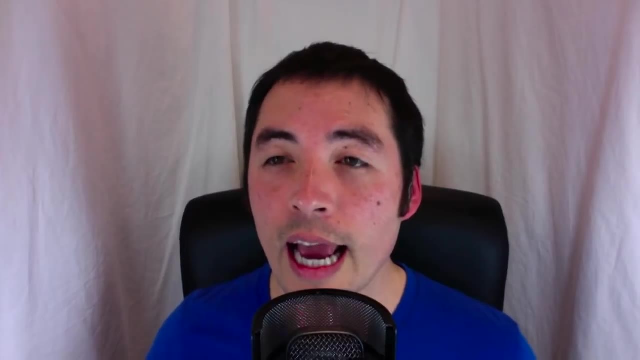 A Practical Guide to Dimensionality Reduction, And it was an awesome presentation. It's a great video, But what I'm going to do is I'm going to pull up his slides on screen and I'm going to briefly go through a couple of his ideas for how you feature selection. 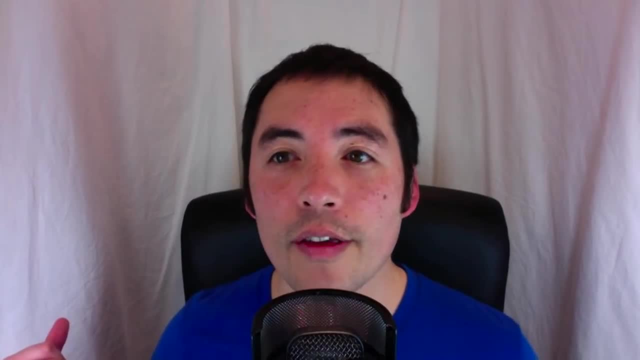 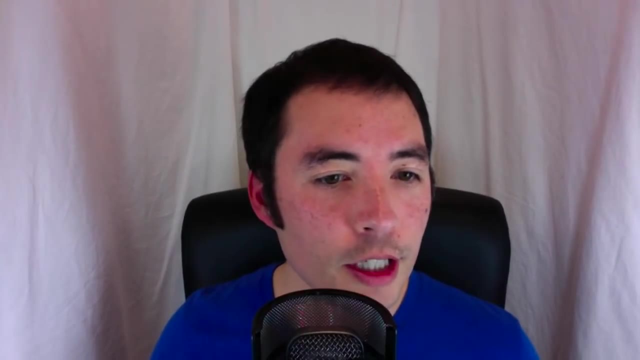 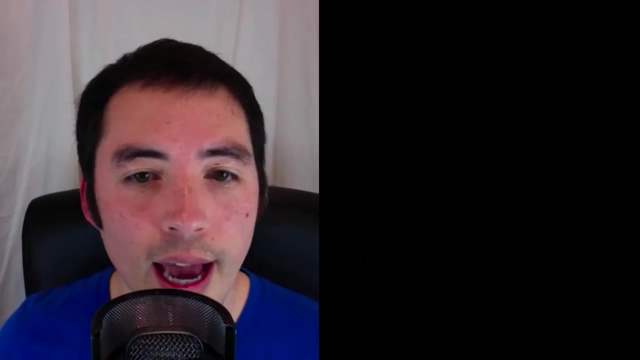 And then I'll talk very briefly about. you know how you do it from a practical level, not just kind of a high level, So it'll take me just a moment. I need to share one of my tabs and let's do that, All right, You should see on screen. 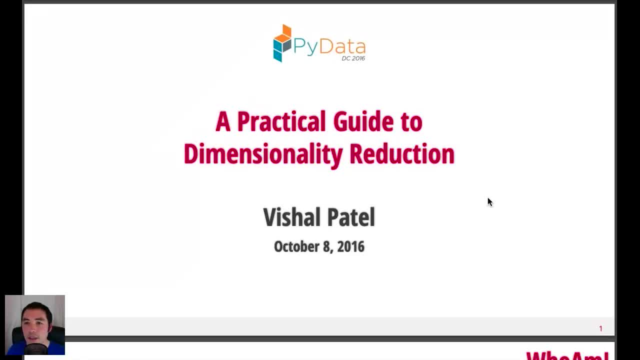 the slides. So it's called the Practical Guide to Dimensionality Reduction, but it's about feature selection, because dimensionality refers to the dimensions of your training data and number of rows and number of columns. So when we're talking about features, we're talking about columns. 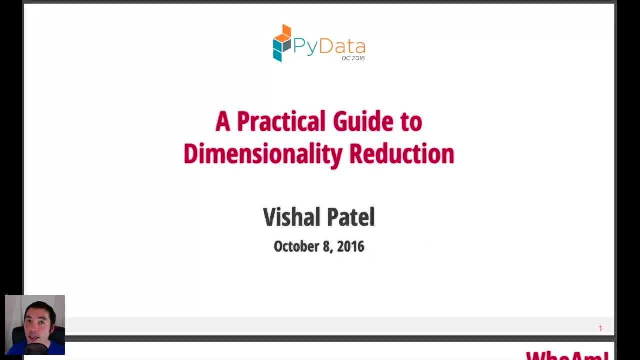 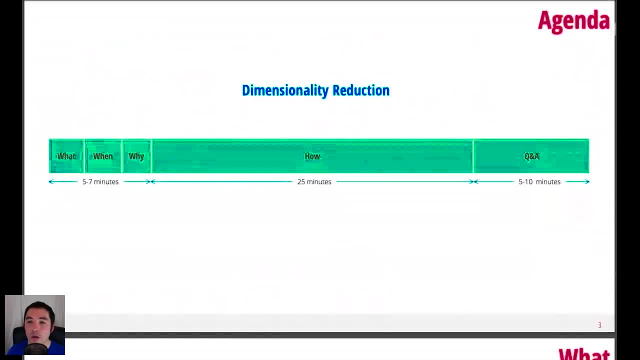 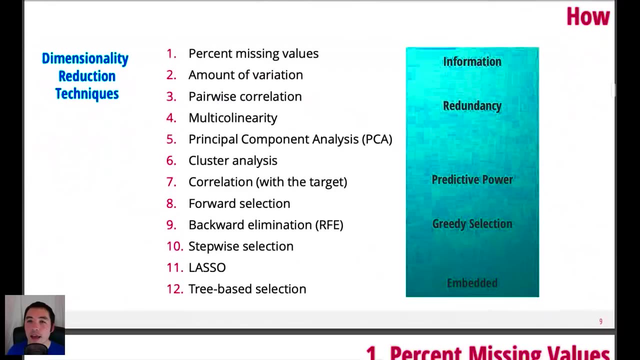 and when we're talking about dimensionality reduction, that means reducing the number of features. Okay, So let me go ahead and scroll down and he has this big list of 11 techniques, 12 techniques, sorry that he uses for feature selection- and I'm just going to. 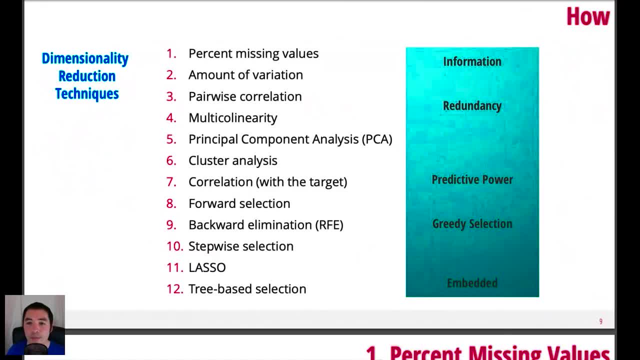 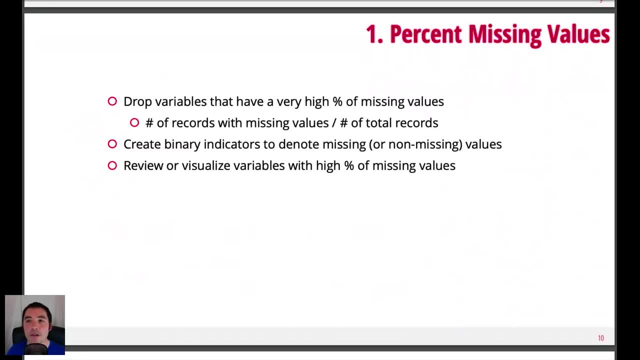 highlight a few of these. Okay, So the first one he talks about is based on percent missing values. So again, Davis has 400 features and he's asking: how do I remove some? And the first idea is to remove features that have a high percentage of missing values. Now, why is that useful? Because features that 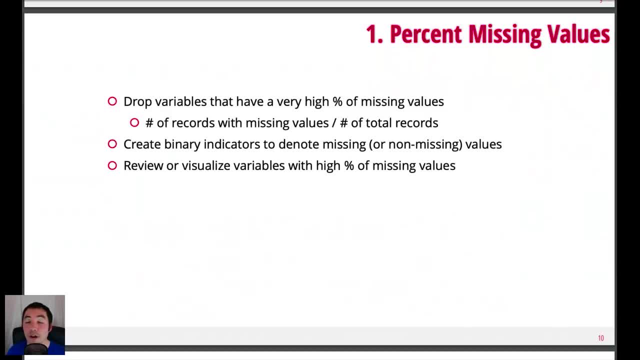 are mostly missing values are not going to be removed. So if you're going to remove a feature from a model, or if you're going to remove a feature that has a high percentage of missing values, well there's another reason that that's going to be removed. The reason the feature won't. 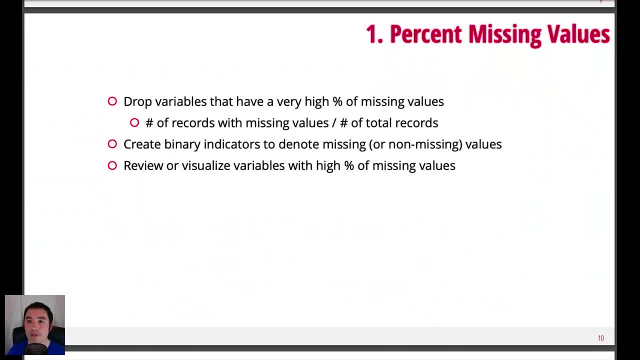 be removed is it's hard to remove small things. Now, what a lot of people might do is they have to go look at the database, look at that and say, hey, what's the row alone in? So, basically, if you're keeping things like�ager, unyielding or calming, you refer to that background. 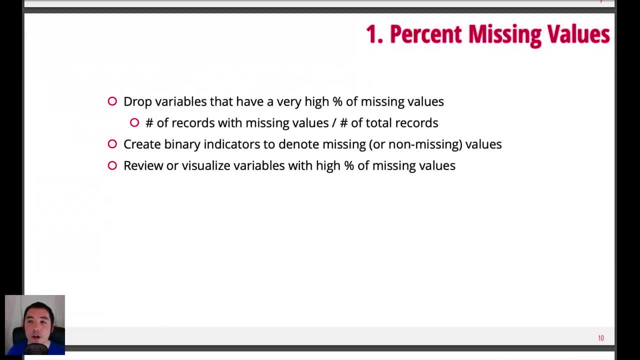 or you refer to the dot line. Now you know that probably won't be removed from any data. Butterfly Sonics is great for paper monitoring and so on, But he says it's not going to be removed. while not onion's a fool, so they have to go to a new one. So the first idea is that what we're 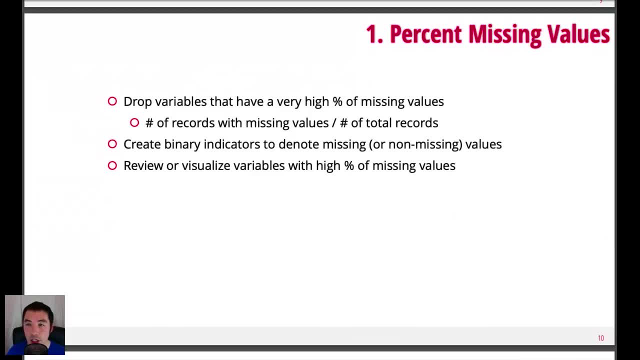 going to do for feature selection. of course, these are two examples of jakles. Because a feature, because well, it might actually be a useful feature, a binary feature of like is missing or not. So even if you're dropping the feature itself, you might encode the missingness. 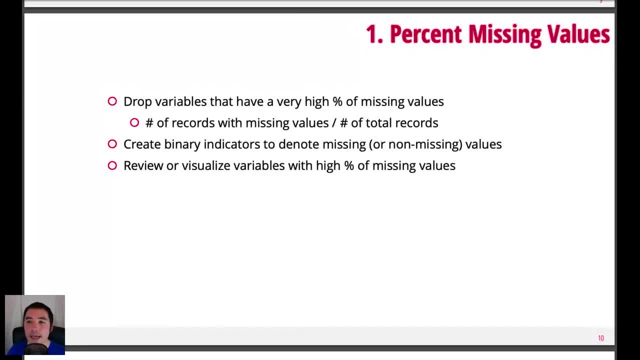 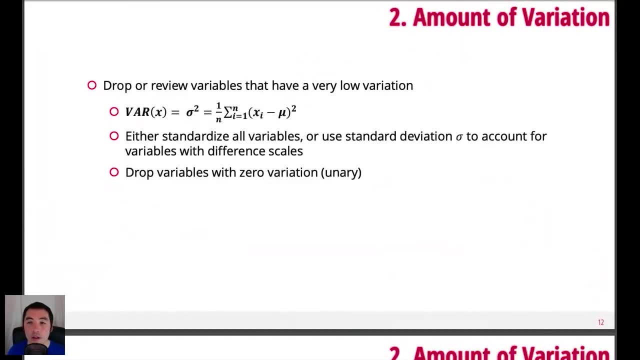 as a feature. Okay, So that's one idea. Next idea: amount of variation. So the basic idea is, if a feature is mostly all the same value, then the model's not going to learn anything from it, So you should drop it. Okay, So that's the next one. Next idea is pairwise correlation. 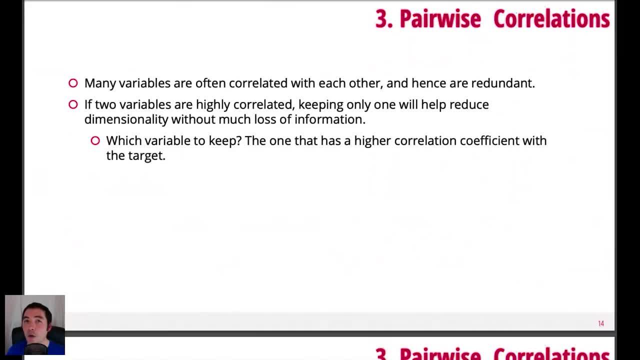 So if two of your features are highly correlated, you can drop one because they're redundant. So if you drop one, you won't actually be losing that much information in terms of what your model can learn from. Okay, So that's another idea. 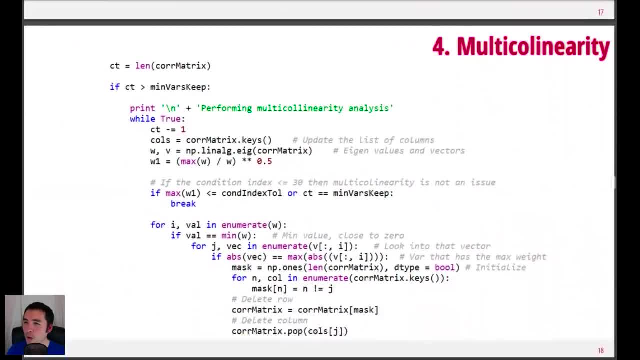 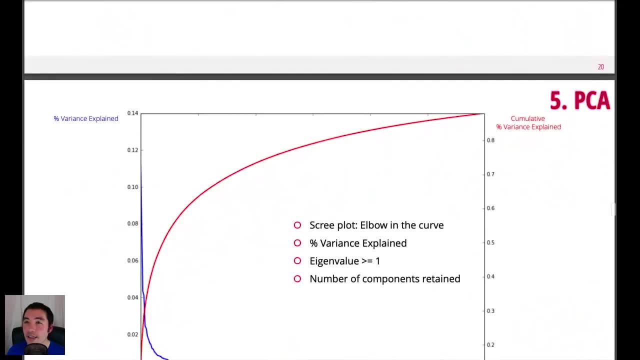 And as I'm going through this, you're probably thinking which ones of these should I do? And I will answer that at the end. I will say that I'm going to provide a lot of ideas, but I'm not going to give you like, here's the one thing you need to do, because there is no one thing. If it was easy, 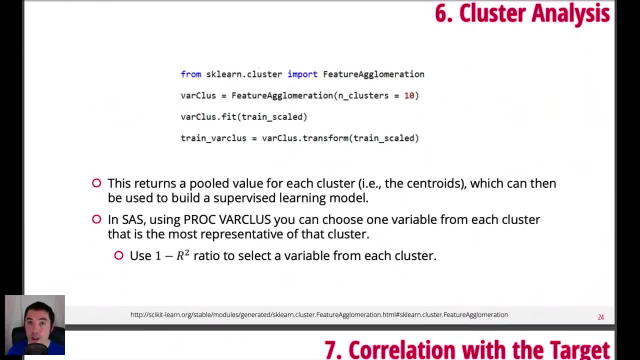 everyone would do it the same way And everyone would just be like: here's what you do And everyone would do it and it would work. But there is no one easy way. There's lots of ideas for how to do feature selection. 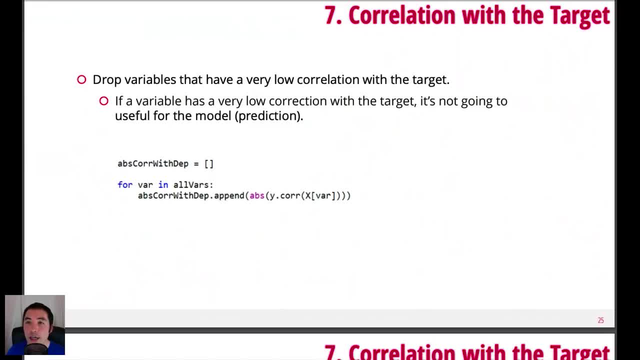 Okay, The next one I was going to talk about is the feature selection. So if you have a feature, selection is correlation with the target. So if a variable aka feature has a very low correlation with the target, then you can probably drop it. Now this might, like any of these techniques can, miss a. 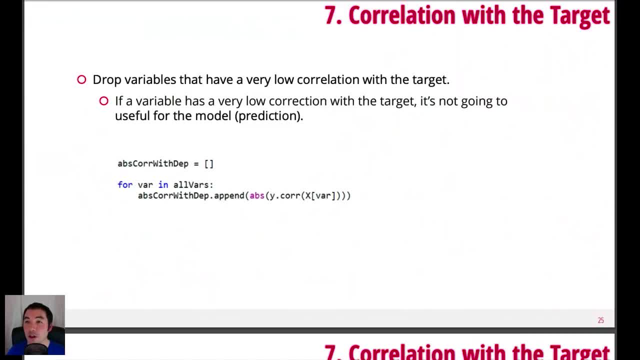 useful feature because there might be a feature interaction such that variable A does not correlate with the target, variable B does not correlate with the target, but variables A and B together. if you turn them into a combined feature, then they are. But there's only so much you can do. You. 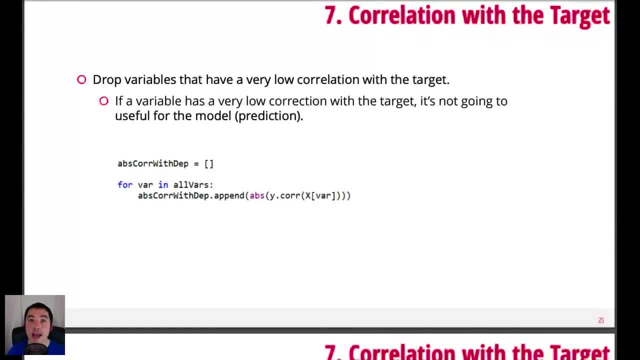 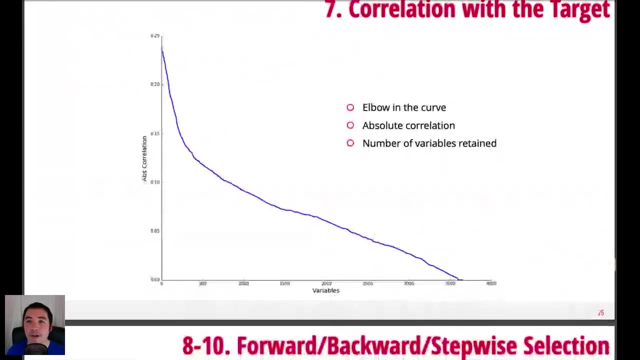 can't, generally speaking, try every possible combination of features, and especially when you have 400 features, So you have to use some sort of technique to do this. Okay, Number eight, nine and 10 talk about forward, backward and stepwise selection And the way forward selection works. 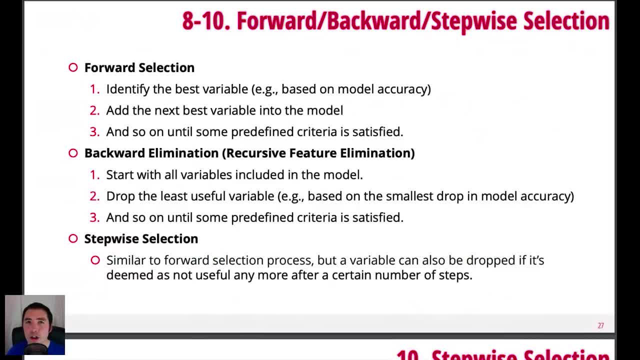 and then I'll talk about the other two- is you start with one feature that you believe to be the best feature and you evaluate. I mean you could actually write a loop, even Just try one feature in your model loop through all 400,. 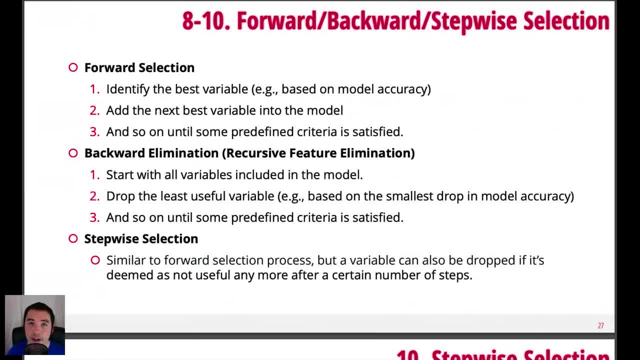 and do cross-validation with the relevant evaluation metric and figure out: okay, here is my one best feature And you add that to your model. Then you try adding a second feature. Which do you add? Well, the best one As determined by some criteria. So you keep doing that until some threshold is met. 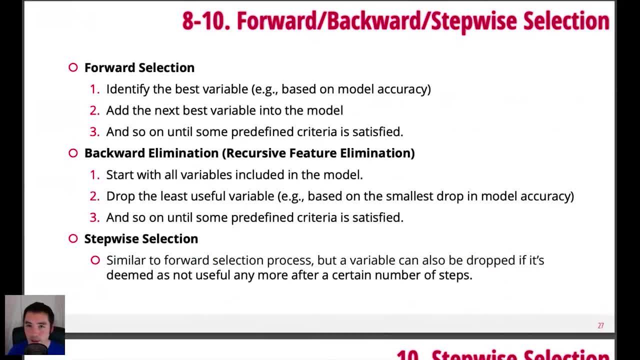 either a certain number of features, you define some performance metric, et cetera, et cetera. Backward selection is essentially the reverse. You start with all of them, You subtract one, You subtract the least important one, And you keep subtracting and subtracting again until 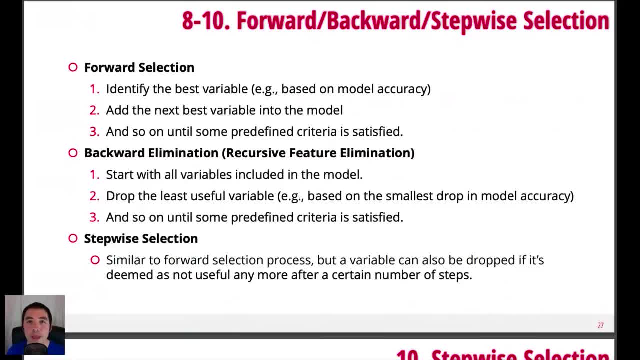 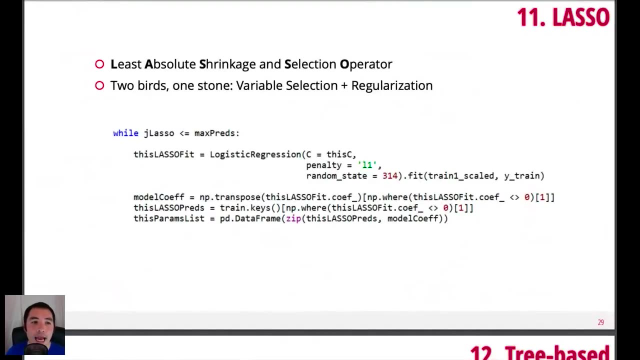 you meet some sort of stopping criteria And then stepwise is kind of a combination of the two. Okay, I'll just have a couple more and then I'll kind of summarize what I've talked about here and provide some other tips. So two more in his recommendations, Lasso- Lasso is actually an 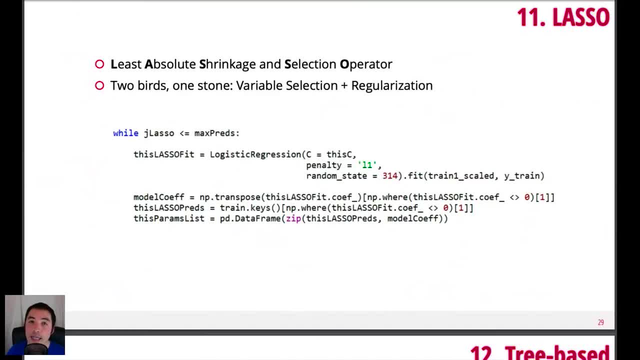 algorithm for creating a regularized linear model. Okay, You may have heard of lasso regression and ridge regression. They're two types of regularized regression. Well, a nice property of lasso is you change this regularization parameter with lasso And like when either the value is really large or really small, I don't remember. 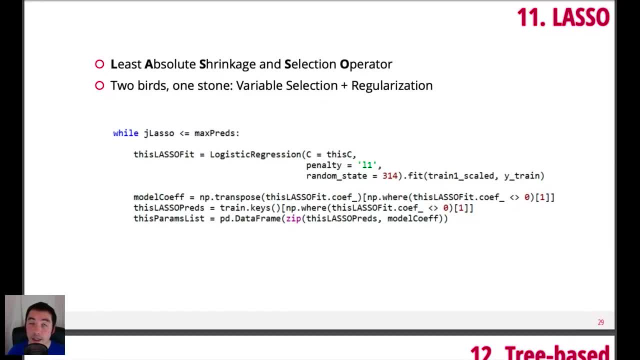 there's no regularization and you just have a plain linear model. Then if you increase or decrease that regularization parameter slightly, then it does regularization which with lasso actually drops. So you can see that it's not a regularization, It's a regularization of the 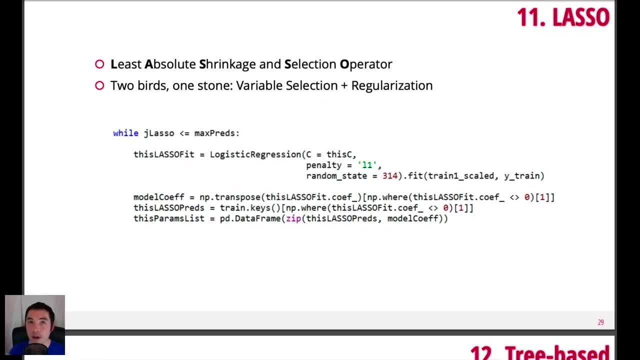 coefficient all the way to zero, And a coefficient of zero means the feature has been dropped. So it essentially does feature selection for you. Now I just said, lasso is for a regularized linear model, A lasso is for regression, but there's regularized logistic regression, for example, that can work. 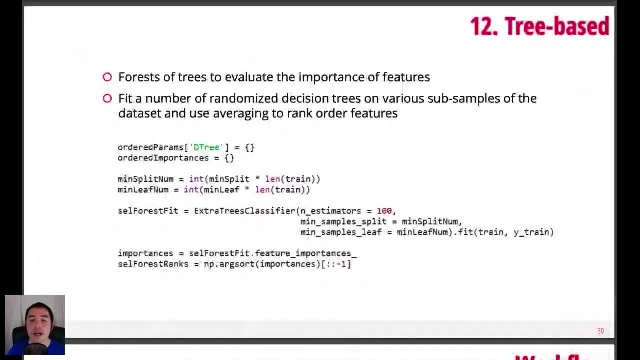 the same way. I think I've said enough about that. The final idea in this presentation is tree-based models And you may know, if you're a theory photographer, you're going to find a lot of tree-based models And you may know that tree-based models are very difficult to learn And you may 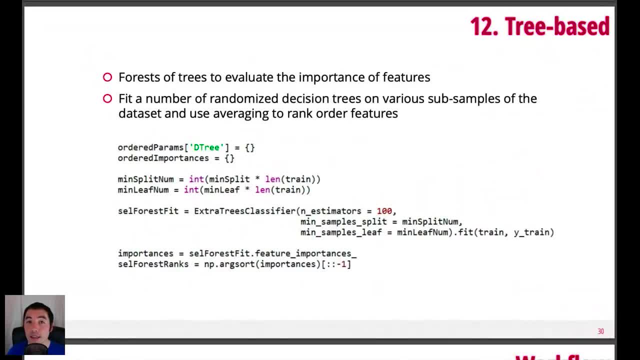 learn that tree-based models are very difficult to learn And you may learn that tree-based models are that with ensembles of trees, of decision trees, such as random forests and other similar models. it automatically computes something called feature importances. You could set a threshold and say: 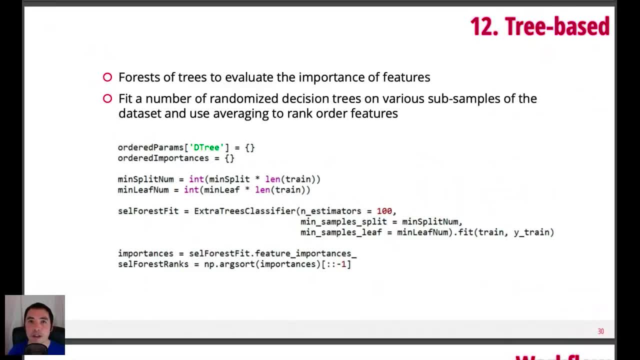 if my model says a given feature's importance is below a certain threshold, then remove it from the model. So that's another idea. These last two ideas are only useful if that is your model that you're using, or you could theoretically use a tree-based model to look at feature importance and 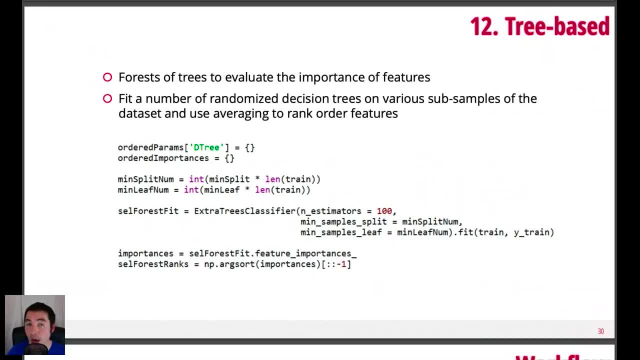 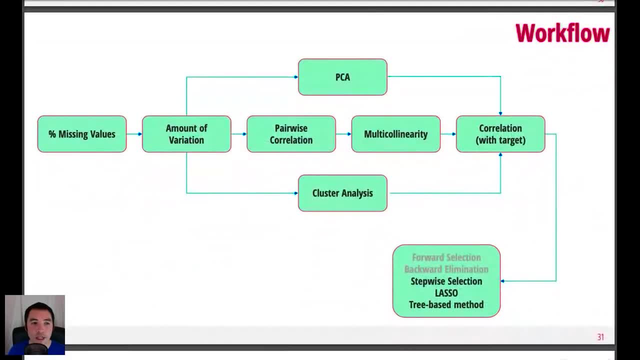 then not actually use a tree-based model for your model that you're building? Okay, so I know that was a lot of ideas thrown at you quickly. I'll just wrap up with some advice and then talk about how to implement this In terms of implementation. Scikit-learn does support some of these. 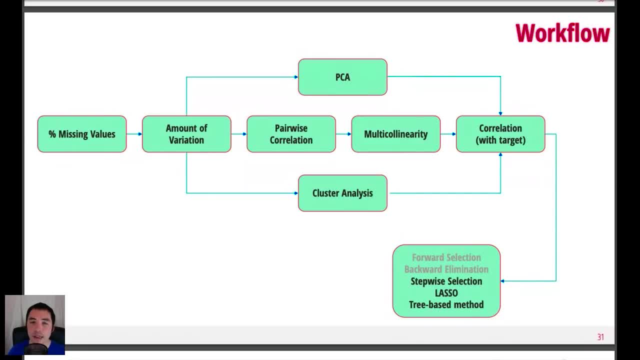 Just sorry. Search for Scikit-learn feature selection or. I'll have a link in the webcast notes And they have a page in the user guide about feature selection techniques they support And many of these are included in some form or fashion. The most kind of I don't know sexy one is forward and backward. 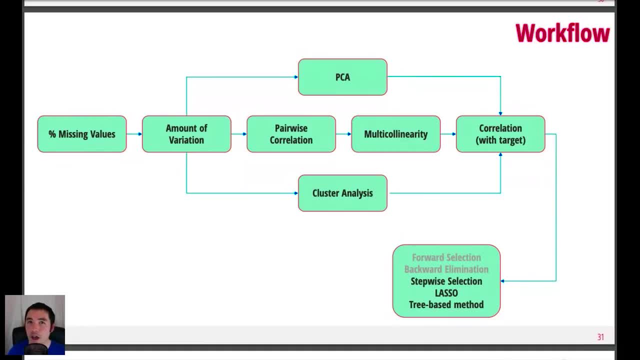 selection because it feels like it's doing a ton of work for you And it is. That's not currently available in Scikit-learn. It is available in a package called ML Extend, and I will link to that in the webcast notes, Though.